which, by the way, I'm going to use the x-intercept right. So, if I'm asking you, here's my equation which, by the way, I'm going to use the x-intercept right. So, if I'm asking you, here's my equation. 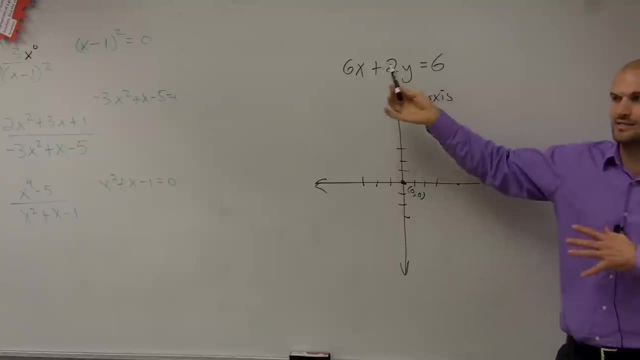 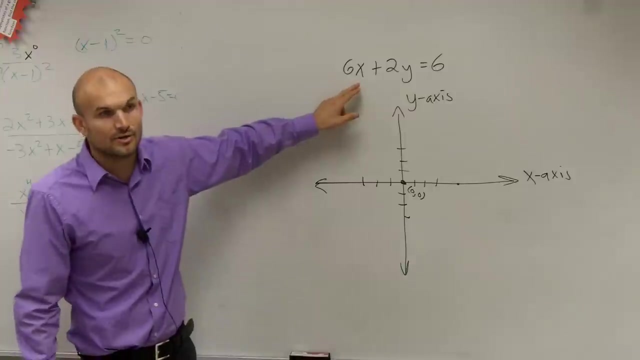 which, by the way, is in standard form. Actually, not really. We could factor out a 2,, but it's in the standard form format. If I say, tell me what the x-intercept is, you don't know what x is right, But do we know what y is? 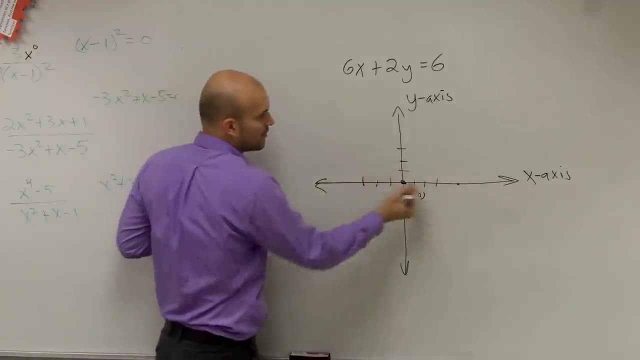 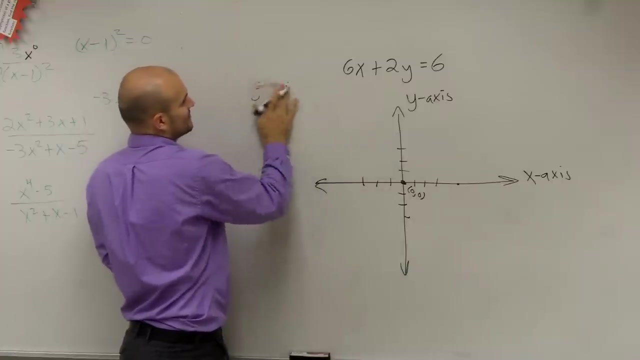 Y has to be what Zero, right? Because I said I don't know where the x-axis is, but no matter what, y is going to be zero. So what we write is: I always like to write two forms. I always 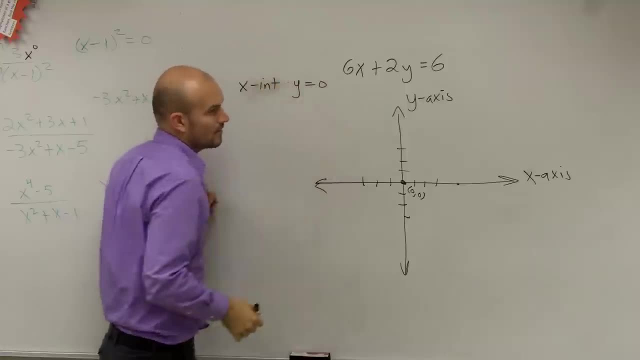 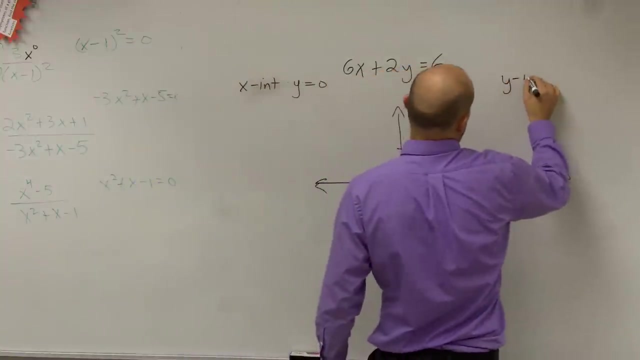 say x-intercept and I say y equals zero, Then what do you think it would be for the y-intercept? What do you think x is on this? y-intercept: Zero. So then I write y-intercept, x equals zero. So we're going to do the problem twice, One for the x-intercept, one for the. 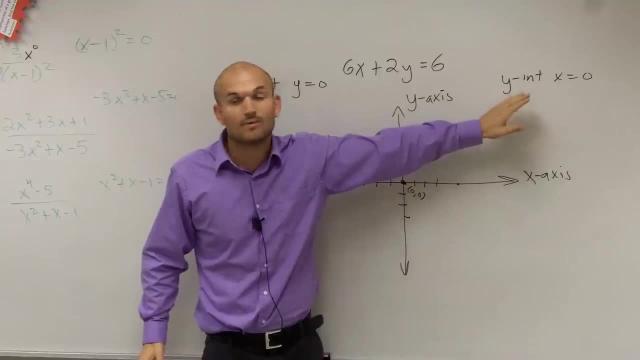 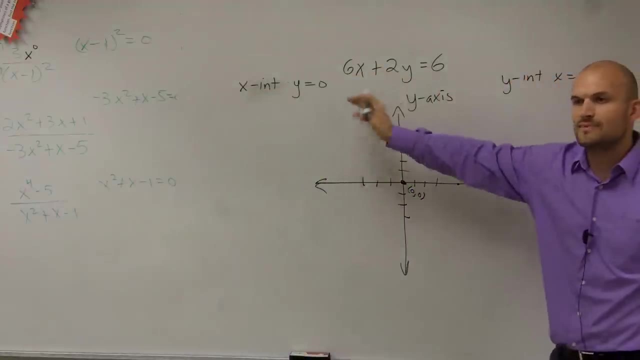 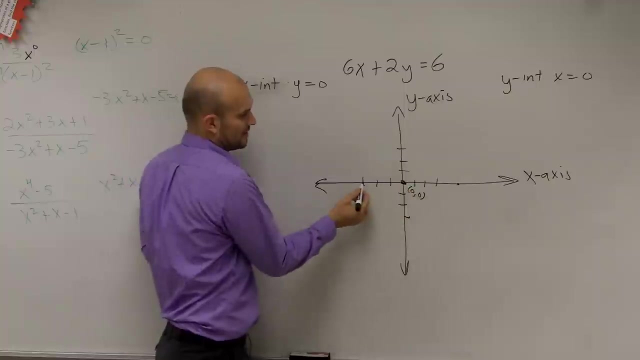 y-intercept, Because that's what I asked you to do. right. Find the x and the y-intercept, Right, Anna? could you please put that away? So what does it mean when y equals zero? We're going to plug zero in for your variable. Y equals zero because, look it, let's pretend. 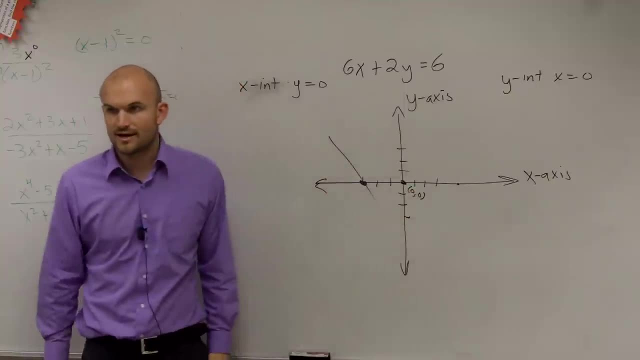 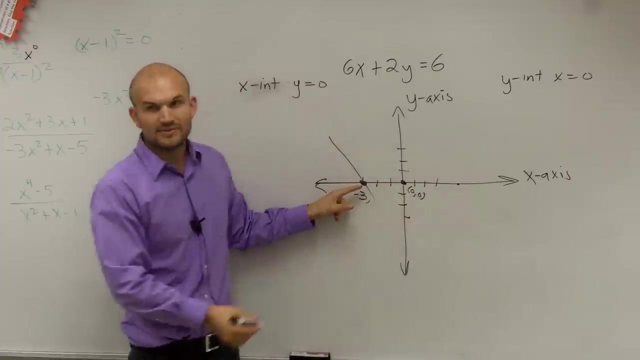 here's my point, right? Let's say, I have a graph Crosses it right there At that coordinate point. right, you had to go over one, two, three. So you went over negative three. but then how high up. 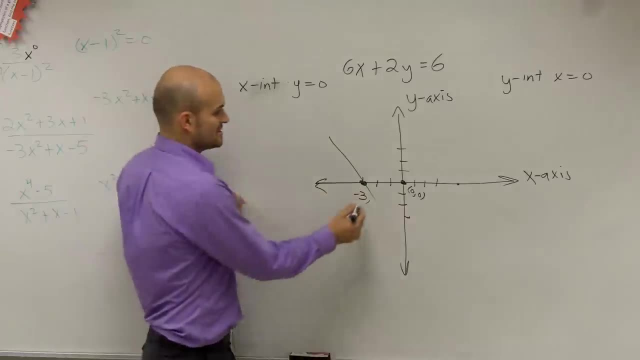 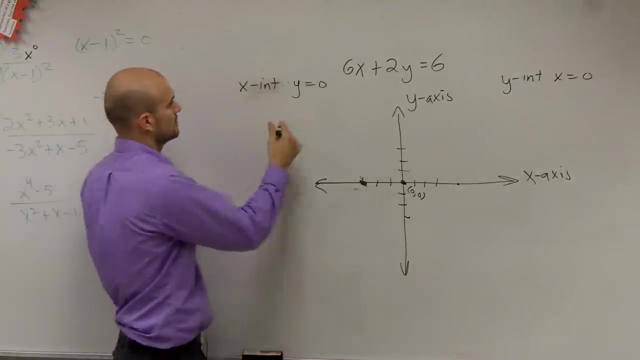 and down. did you go on the y-axis? You didn't go anywhere, right? So it's negative three comma zero. Does that make sense? Okay, Now Teachers, pardon the interruption. I do have some bus changes to announce today. 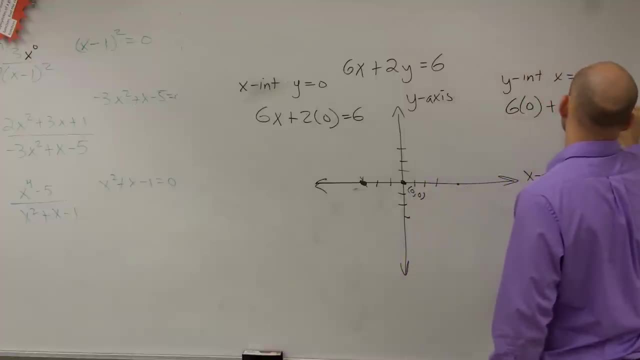 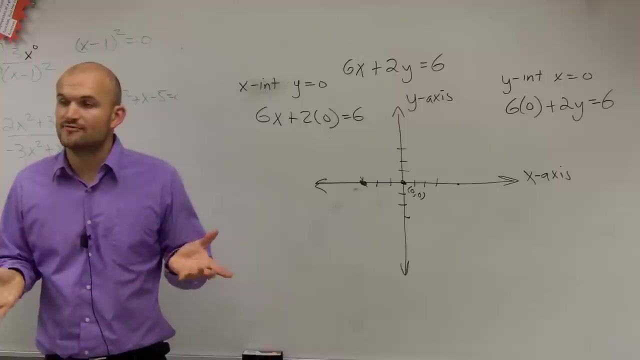 Students who ride bus 612 will ride bus 531 today. It will be a late bus, So we ask that the students on bus 612 wait on the bus. You use this to find the x and where it crosses the two axes and then connect. 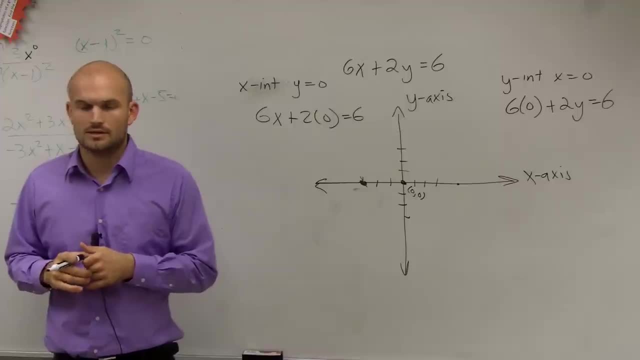 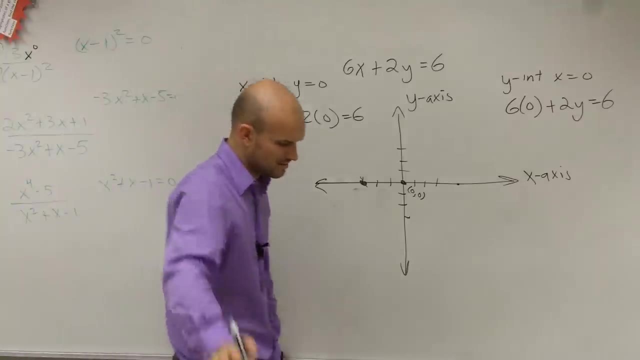 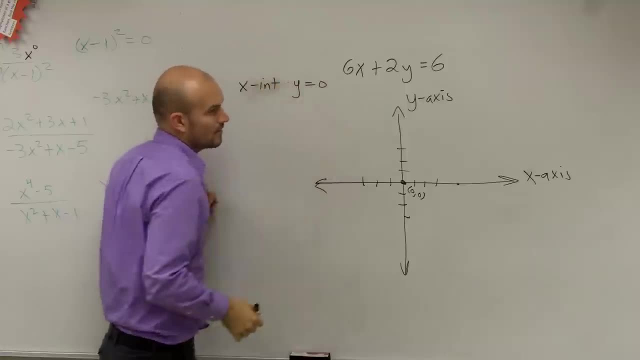 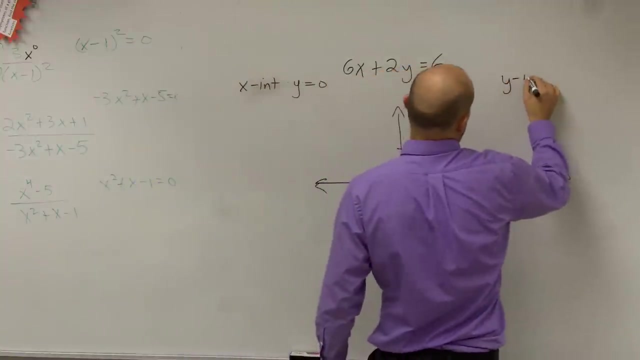 say x-intercept and I say y equals zero, Then what do you think it would be for the y-intercept? What do you think x is on this? y-intercept: Zero. So then I write y-intercept, x equals zero. So we're going to do the problem twice, One for the x-intercept, one for the. 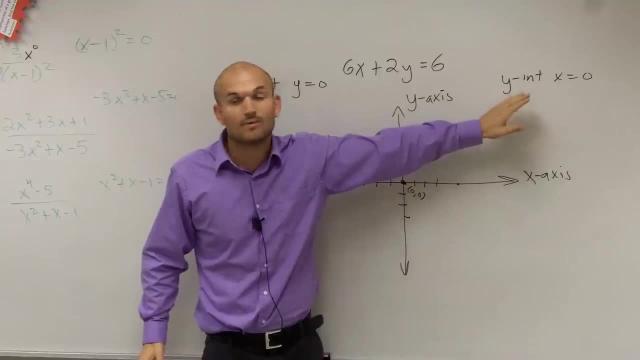 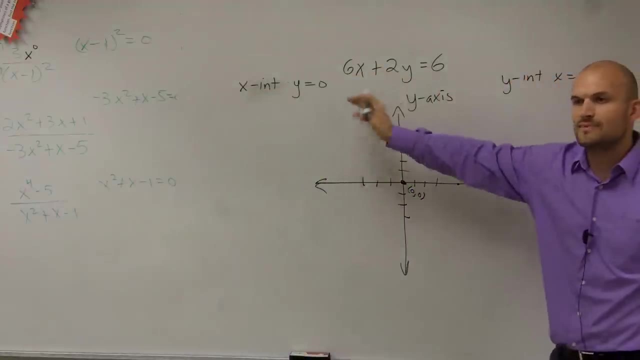 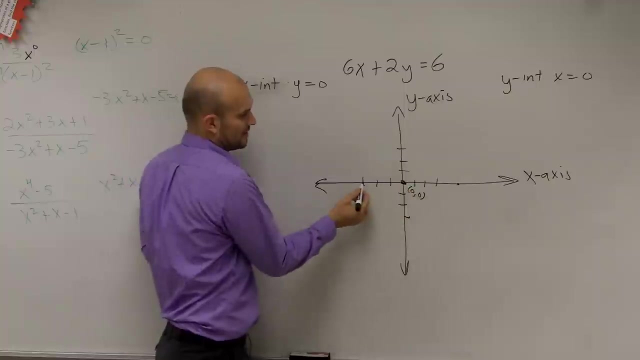 y-intercept, Because that's what I asked you to do. right. Find the x and the y-intercept, Right, Anna? could you please put that away? So what does it mean when y equals zero? We're going to plug zero in for your variable. Y equals zero because, look it, let's pretend. 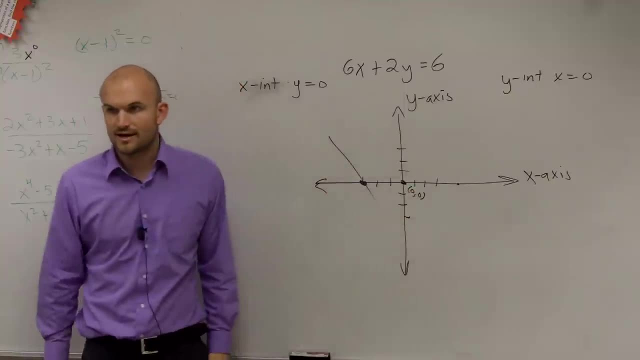 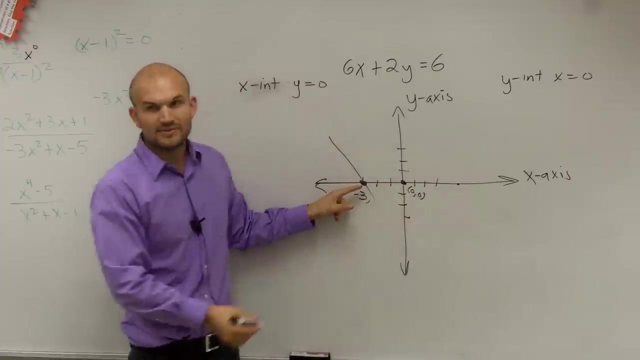 here's my point, right? Let's say, I have a graph Crosses it right there At that coordinate point. right, you had to go over one, two, three. So you went over negative three. but then how high up. 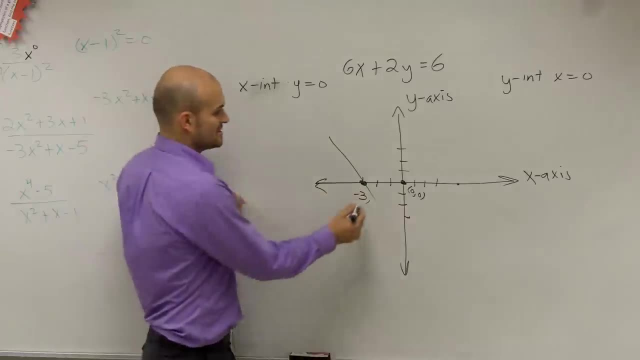 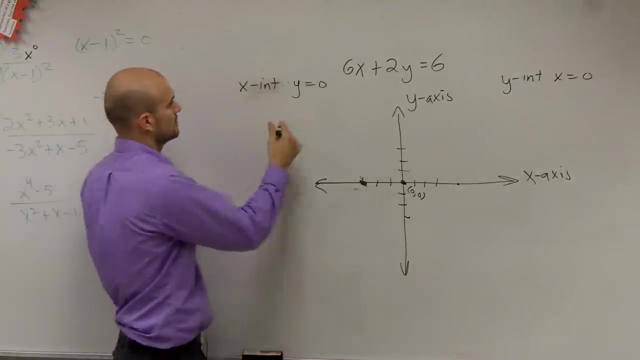 and down. did you go on the y-axis? You didn't go anywhere, right? So it's negative three comma zero. Does that make sense? Okay, Now Teachers, pardon the interruption. I do have some bus changes to announce today. 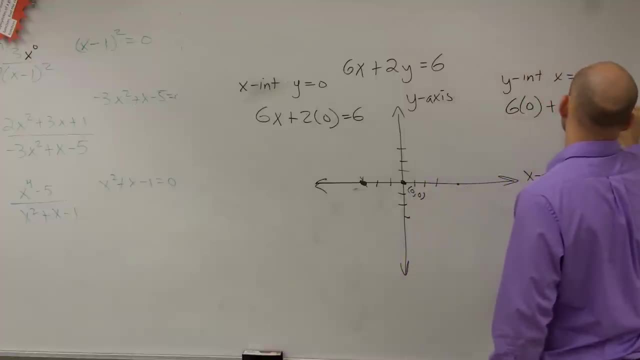 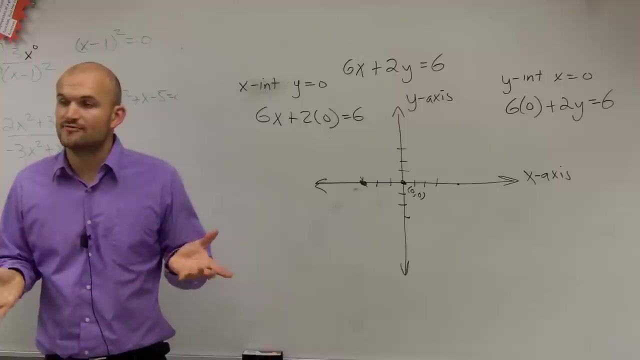 Students who ride bus 612 will ride bus 531 today. It will be a late bus, So we ask that the students on bus 612 wait on the bus. You use this to find the x and where it crosses the two axes and then connect. 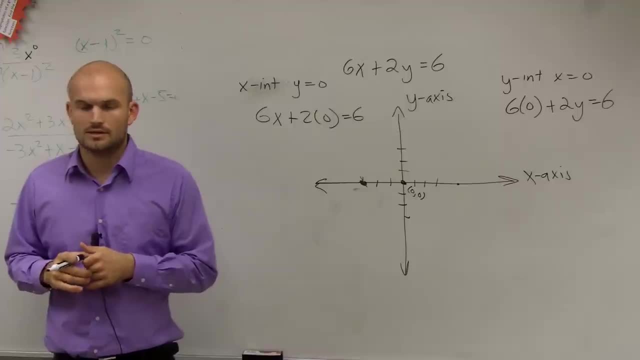 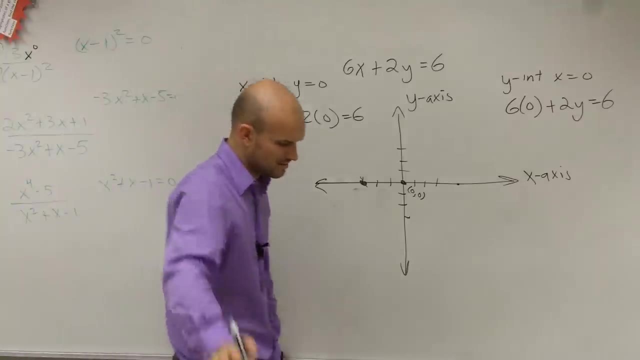 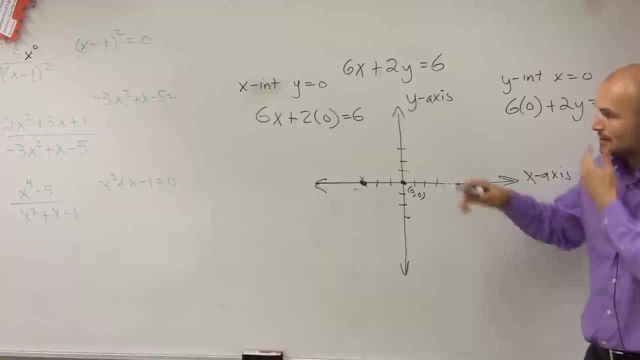 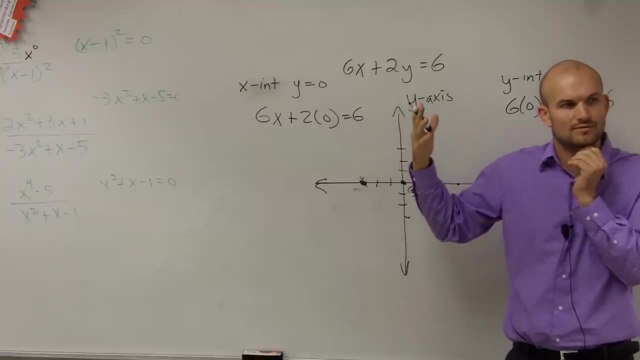 Okay, So not done here yet, Cedric. So, ladies and gentlemen, remember, at each y-intercept or x-intercept, the other value is equal to zero. Can we hold off, ladies and gentlemen, Catherine? Yes, So now what we're going to do is plug zero in for x and solve What's two times zero. 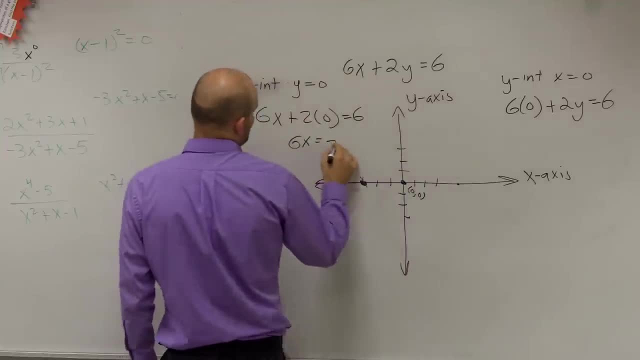 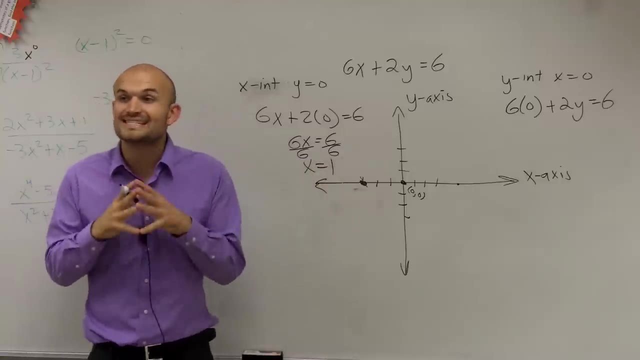 Zero, Zero. So I'm left with 6x equals six. Divide One, Y always equals zero. for the, The x-axis- I'm sorry, the x-intercept- Whenever you want to find the x-intercept- y equals zero. 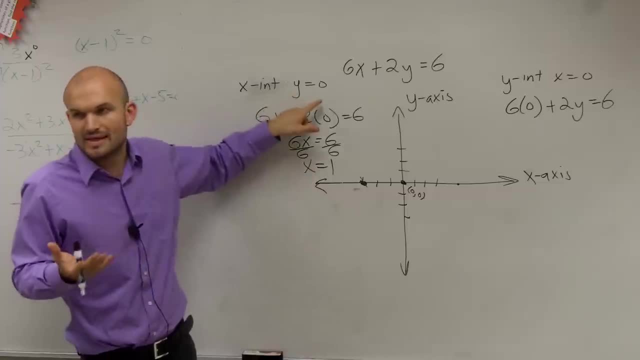 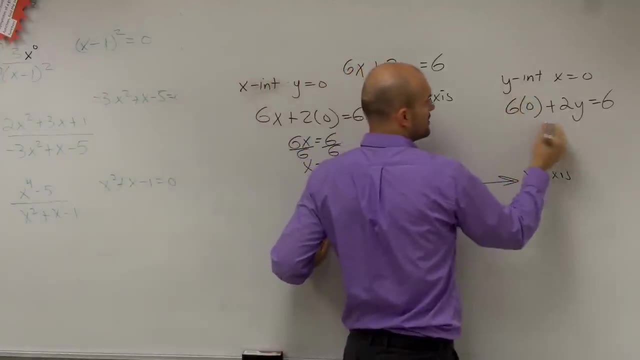 How do you know it's the x-intercept. Well, that's what we're trying to find. That's the problem. it's asking is find the x-intercept. Now, to find the y-intercept, you plug x equals zero, That's equals zero. So you have 2y equals six.